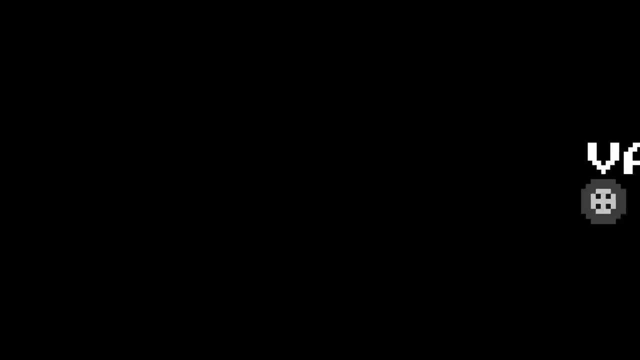 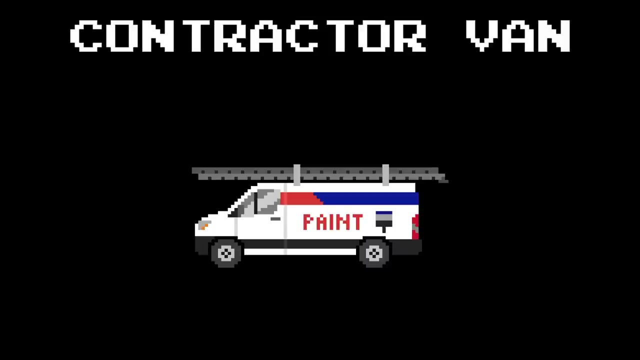 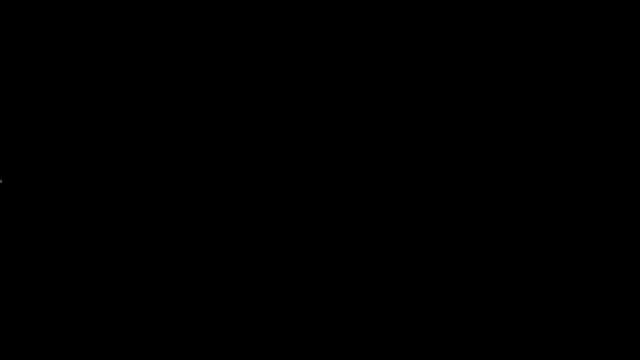 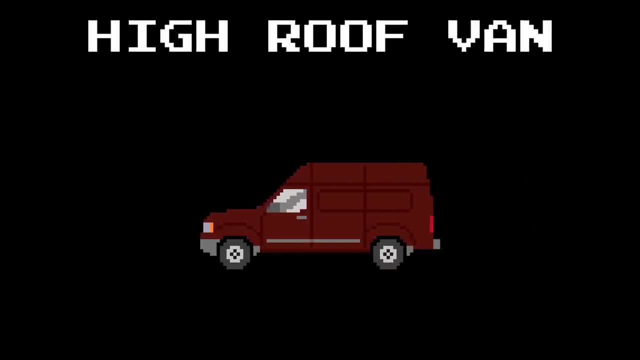 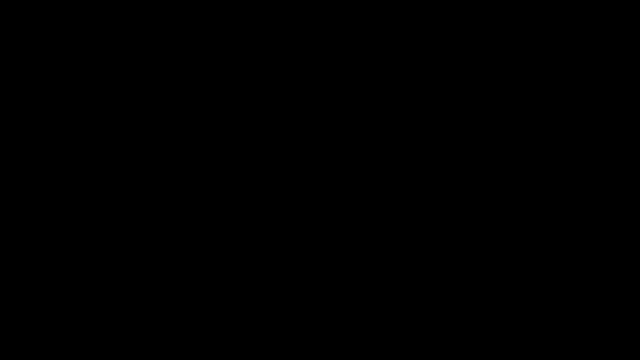 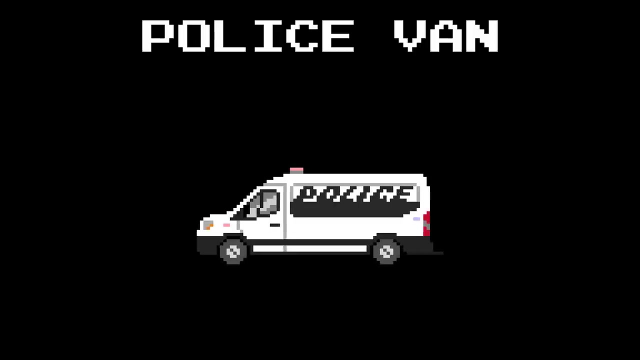 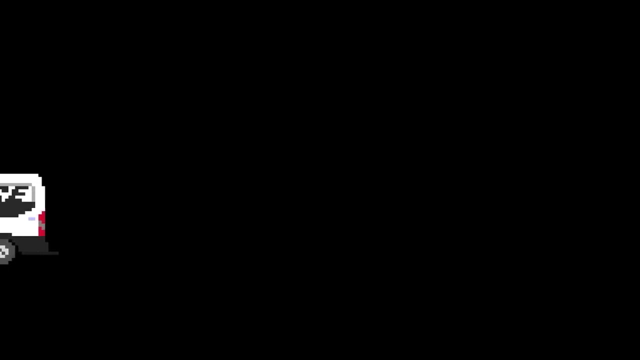 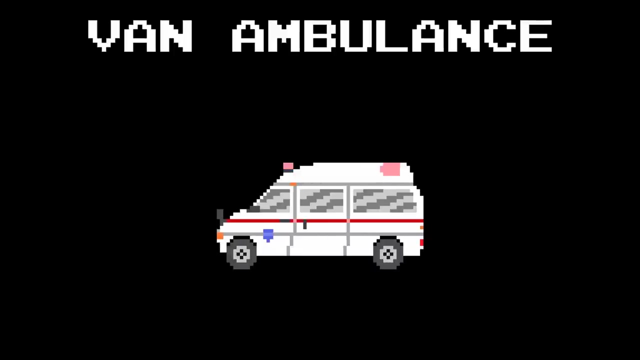 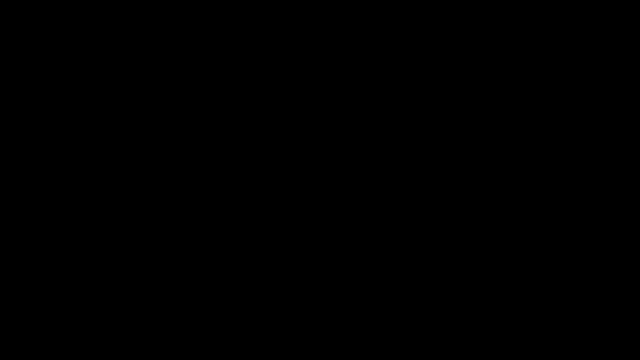 cargos, vans cargo van passenger, van contractor van high-roof. van minivan. minivan minivan taxi. minivan taxi refrigerated. van minivan taxi, minivan taxi fire. van minivan taxi, minivan taxi Police. van Van ambulance Compact. van Microvan. 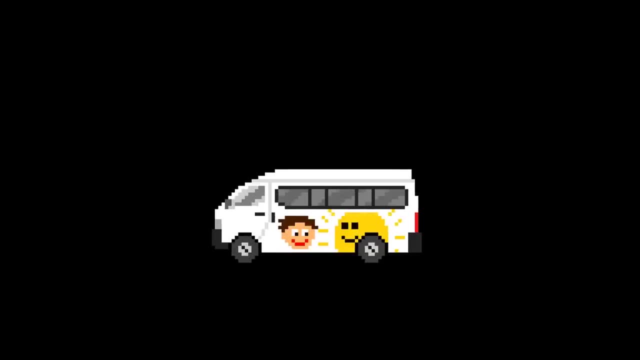 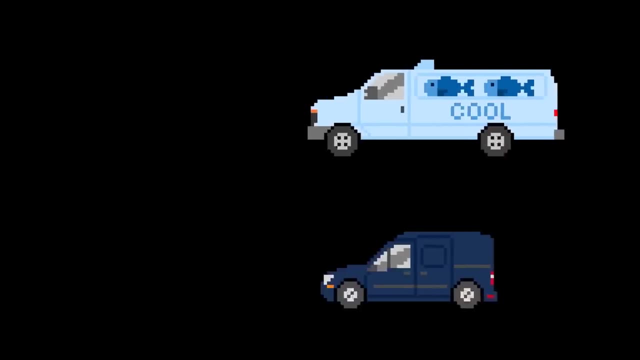 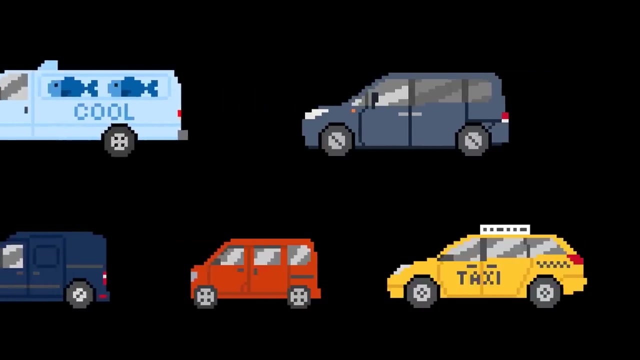 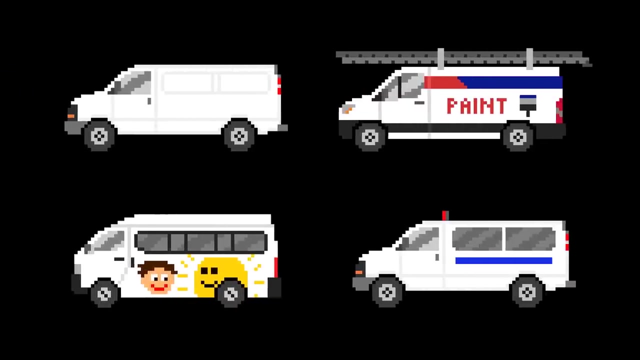 Preschool van Small group van Van de Linde, van de K Nueve, de Areia, van de Lique to Connect to frustrate the small group van van van de Linde, van de K Nueve, van de stbe van van in theekda.